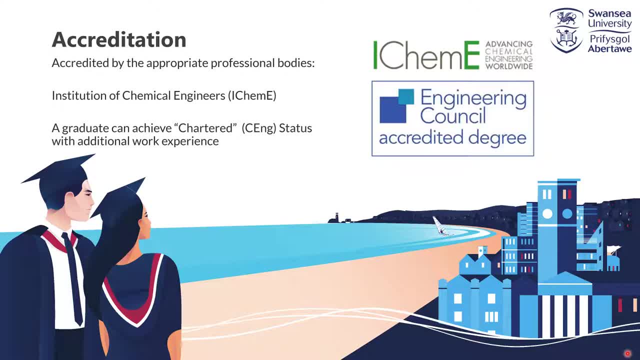 by the Institute of Chemical Engineers and the Engineering Council. These are the professional bodies that we are expected to work under. As long as you graduate with an accredited degree, you can then work on trying to obtain chartered status, which means that you are 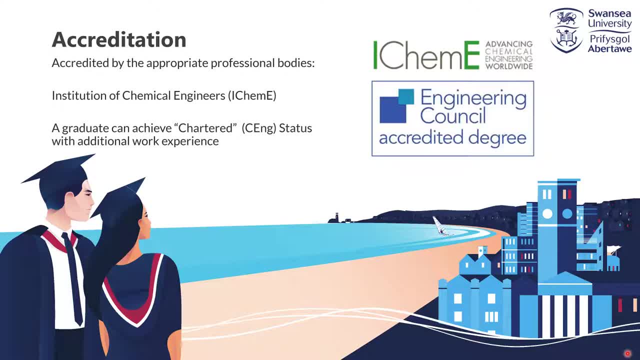 a chemical engineer at the top of your professional game, so to speak. This comes through additional work experience, and what you will find is the companies that you will be working with after graduation will tend to put you on schemes or put you in working on projects. 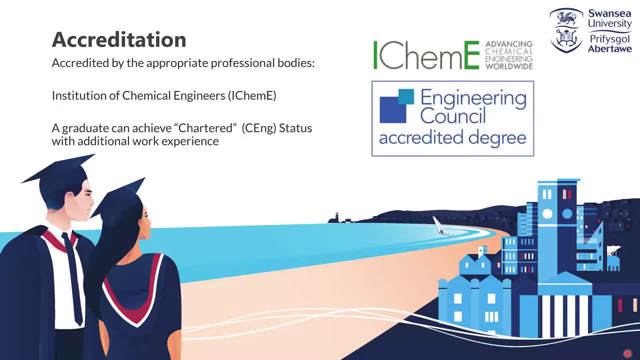 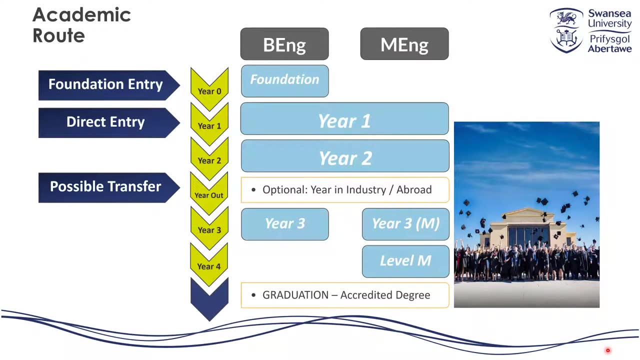 And things like that, which will give you the additional work experience you need to achieve chartered status, And there is an expectation that you will try to work towards gaining this status. So let's have a look at the academic routes. We have two academic 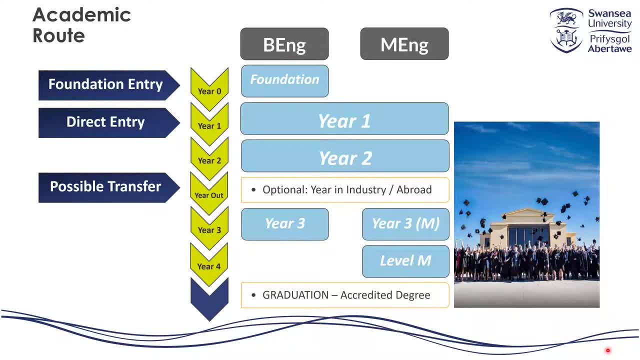 routes here at Swansea University: the bachelor's in engineering- B Eng and the master's in engineering- M Eng. Now both the B Eng and the M Eng share the B Eng and the M Eng, and both the B Eng and the M Eng share the B Eng and the M Eng. 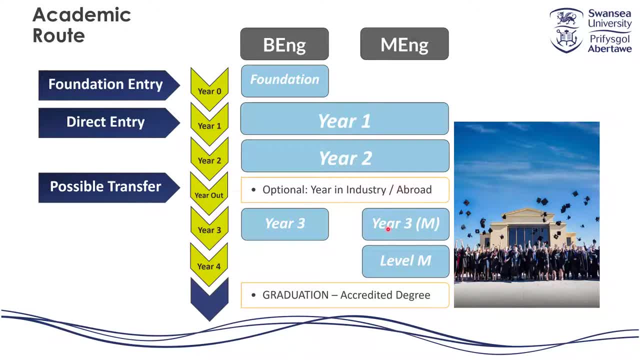 Now both the B Eng and the M Eng share the B Eng and the M Eng. Now both the B Eng and the M Eng share. the B Eng and the M Eng share the same first three years of the course. So you come in, you do year one, you do year two, you then have the. 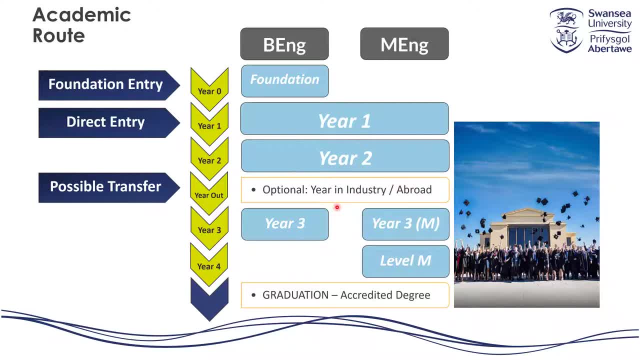 option to take either a year in industry or a year abroad and then come back and complete year three. If you don't take this year out on the B Eng, you just do year one, year two straight to year three And then you can graduate with an accredited B Eng. 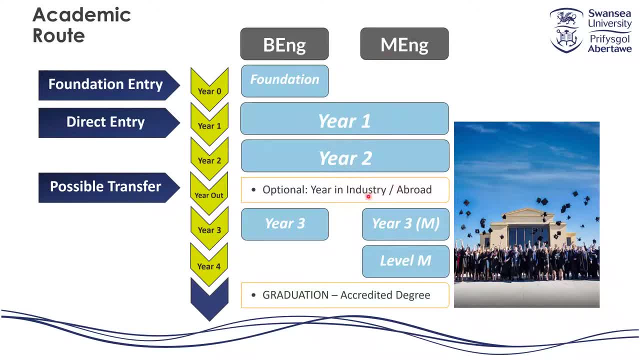 On the M Eng. if you don't want to take the optional year in industry here after year two, you may decide to do it after year three instead. That is an option available to you. What we tend to find is students who are on the M Eng scheme prefer to do this because 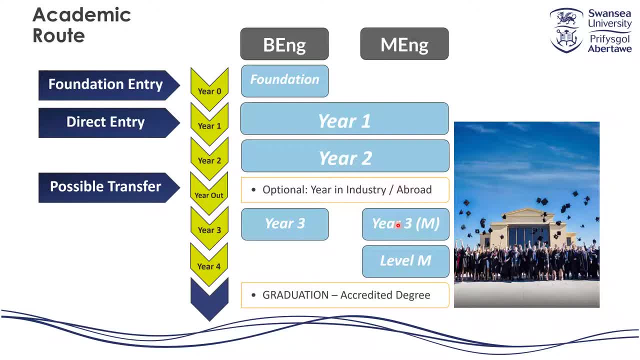 you'll have done the third year design project and you'll have more advanced knowledge which will allow you to work in more advanced projects for the company that you're working for. So it's a great opportunity that you're working for in a year in industry setting. 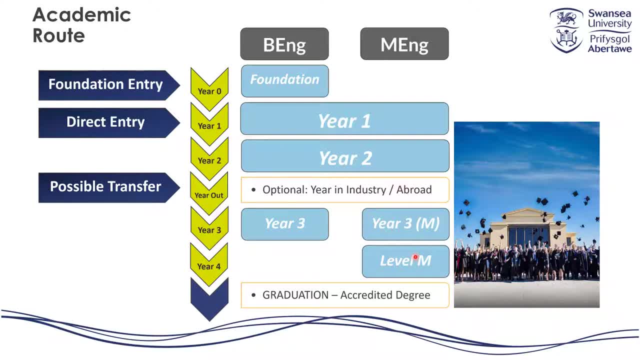 The other part to the M Eng is level M. So this is the fourth year if you're going straight through without any year in industries or year abroad, or the fifth year if you've taken an optional year out for a year in industry or year abroad. 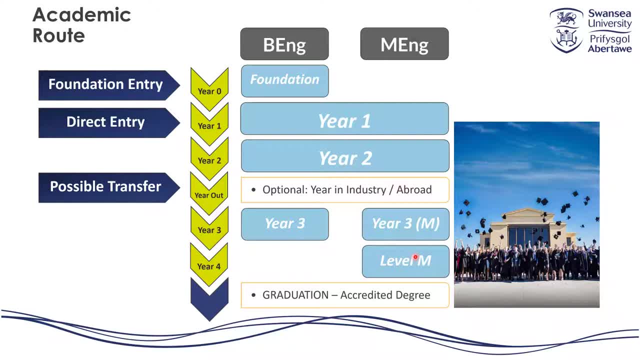 Now, one thing to mention that is unique to Swansea is that in the M level there's a module called the M Eng. We have an industrial research practice module. This module means that you do a two day a week internship, either working with a member. 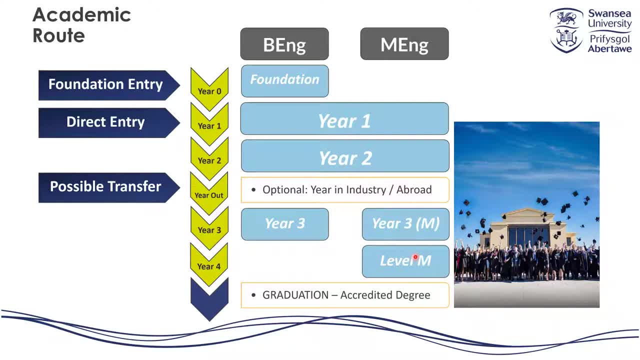 of staff at the university on a research project at the university. This could be working in collaboration with existing projects Or Collaborating, Or collaborating with some external sponsors. The other option that you could be doing is a two day a week internship, working for 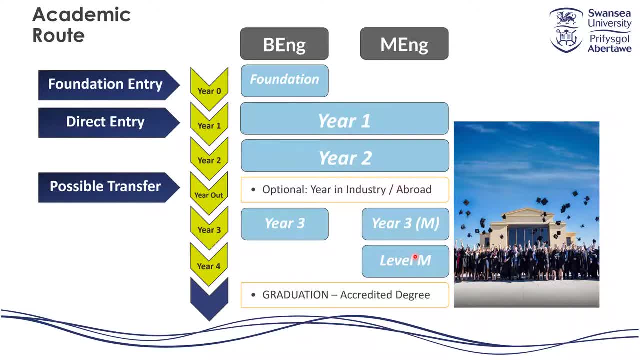 a company in the South Wales region. So if you've taken the option to do a year in industry earlier in the scheme, you may decide that you would like to gain some research practice and decide to do your two day a week internship with Members of staff. 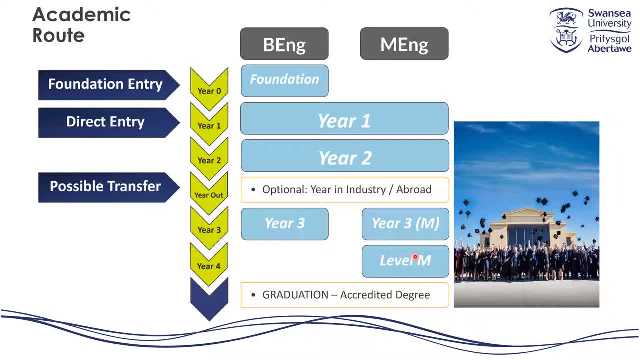 Okay, If you didn't take out a year in industry option, it's an opportunity for you to gain some industrial practice by choosing to take a two day a week internship with a company in the South Wales region- Okay. Other thing to know is it is possible to swap. 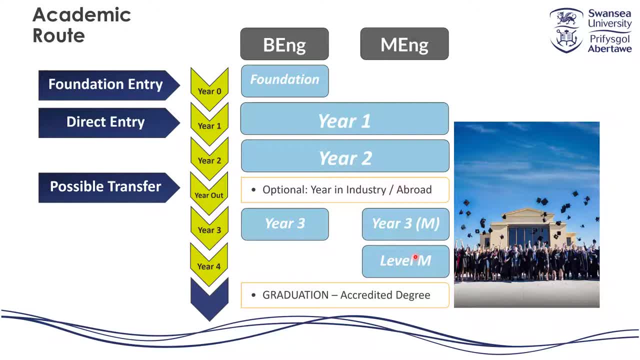 Between the degree schemes. if you've come in on the BEng, there are opportunities in the first two years for you to transfer up to the MEng Okay, And similarly, if you don't meet the requirements to stay on the MEng, you may be asked to transfer. 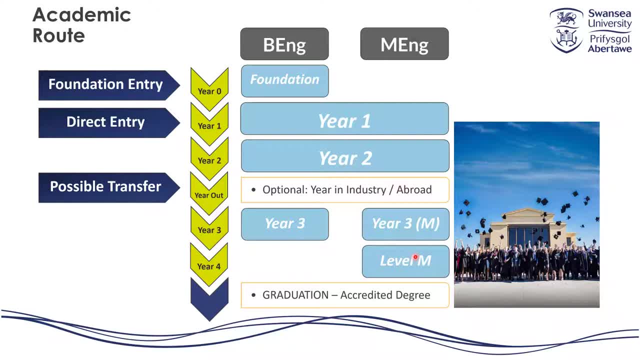 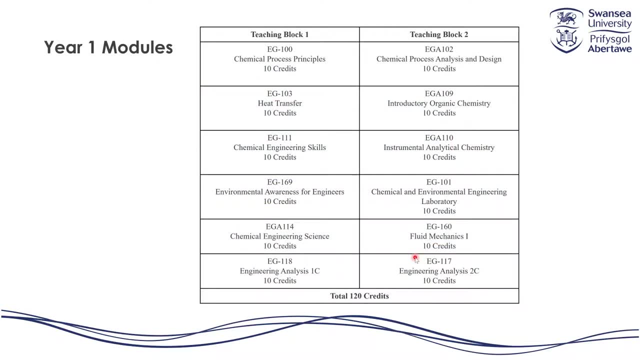 back down onto the BEng. Okay, Thank you. Bye, Bye, Bye. So let's just have a little look at what you might be looking at in the first year of study here. Okay, our course has an emphasis on teaching you the theory and the fundamentals at the 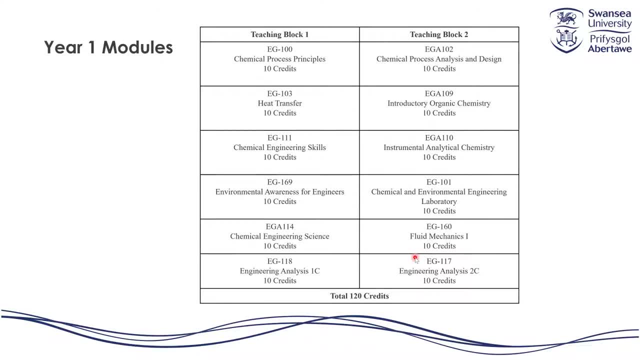 start and then getting you to apply them in the second half of the year. So in the first half of the year we'll teach you all the fundamentals of chemical process. principals Had metaphorical concepts for funding at the beginning, energy balances and things like that. we also teach you heat transfer. we have a chemical 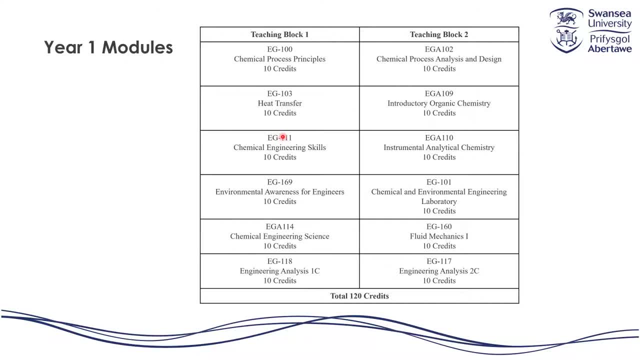 engineering skills module where you learn about cad work, update your skills on using excel and word to a professional standard. we also have a module here on environmental awareness for engineers and things like that. we've also got chemical engineering science, which brings in some more the mass transfer and the thermodynamics that you need to learn, and we have a maths module. 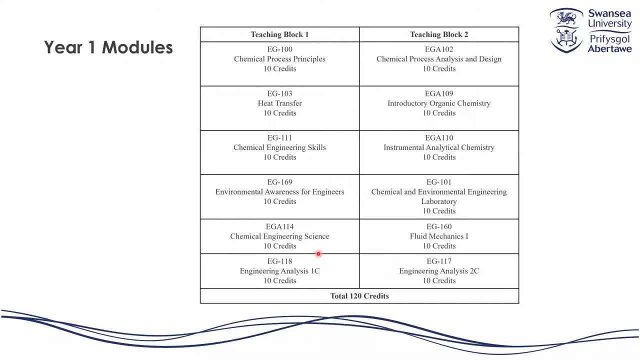 in engineering analysis 1c and then what you find in the second semester of the two of the year. in teaching block two we have chemical process analysis and design, which is a small design project module that you do in the first year or you put into teams and you have to crack. 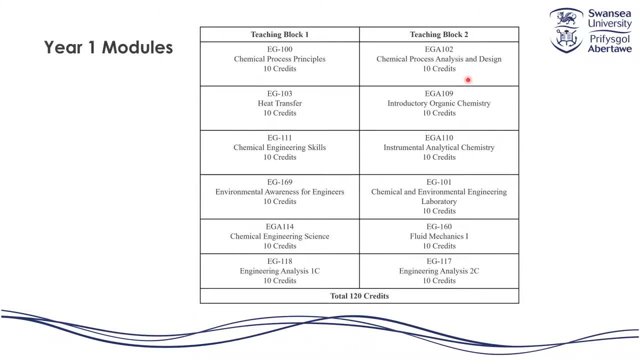 a problem that we've set. usually it's based around the process and it involves you utilizing the skills you've learned in chemical process principles, chem and science, chemical engineering skills, heat transfer and environmental awareness- to to crack the problem and produce a report and an analysis of your findings. okay, you're going to be involved in. 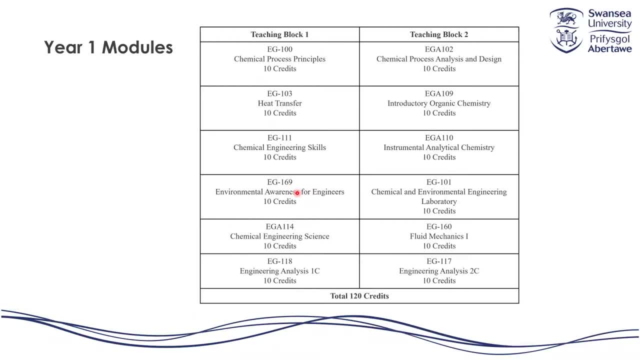 doing presentations, writing reports, things like that. we also have two chemistry modules, one on inorganic chemistry and one on analytical chemistry, to make sure you've got all the necessary chemical chemistry understanding that you require as a chemical engineer. and then we have the chemical and environmental engineering laboratory where you are doing experiments based on. 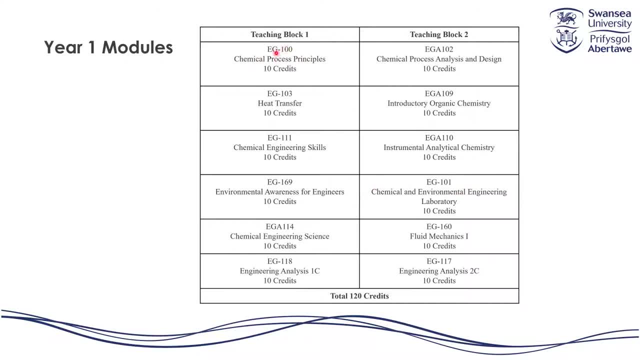 the fundamentals that you've learned in chem: process principles, heat transfer, chem and science. fluid mechanics one. yeah, you're going to be doing practical experiments to reinforce your learning of those chemical engineering fundamentals. as i mentioned, there's a fluid mechanics module here, so i'm going to be introducing you to flow of fluids through pipe works: pressure differences. 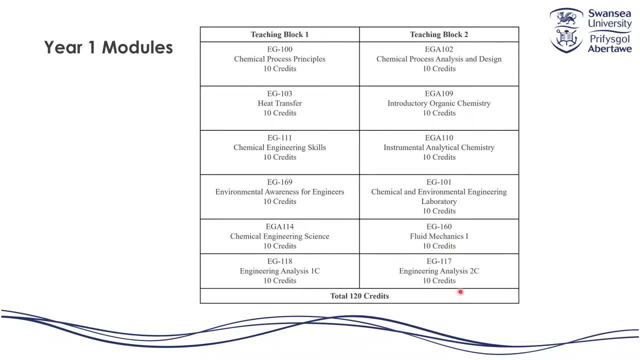 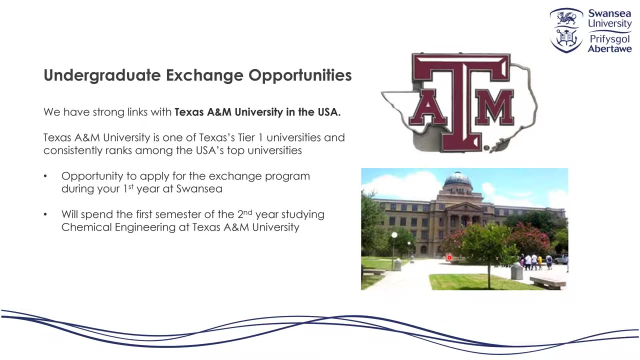 things like that, and then we also have an additional maths module that teaches you some of the more advanced mathematics that you need to know as an engineer. we do have undergraduate exchange opportunities here at swansea university. we have very strong links with texas a m university in the united 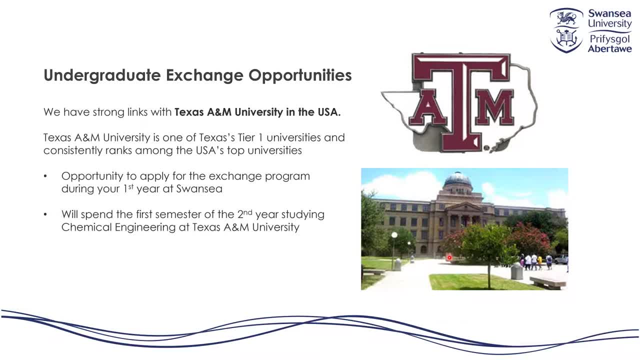 states. it's one of texas's tier one universities and consistently ranks among the usa's top universities. there's an opportunity for you to apply for this exchange program during your first year at swansea university. it's all based on your grades in the first semester. ideally, you need to. 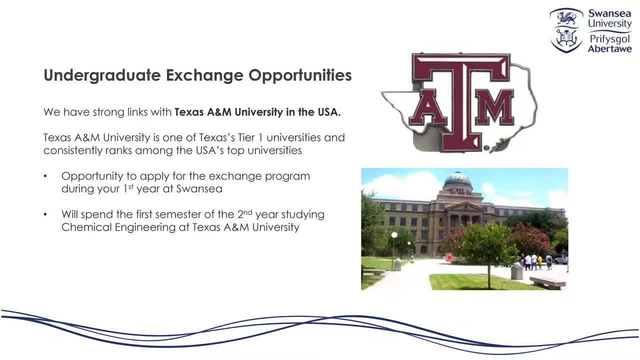 be averaging first class and we tend to only send a very small number of students on this course. but if you are successful in this exchange program, you will spend the first semester of the second year studying chemical engineering at texas a m, doing the same modules there that you would have done. 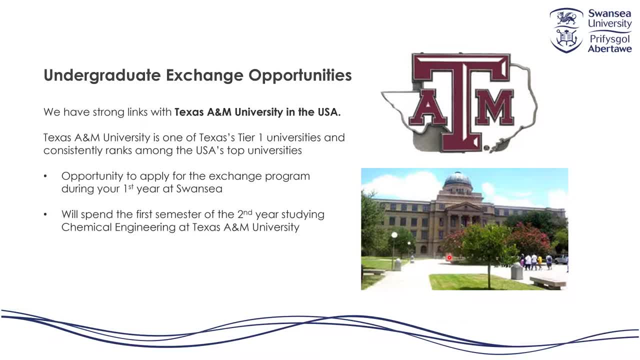 here at swansea university, but you will be learning them under the united states education system, so be doing comparable modules to what you would have done with us over here. so you'll be going out in august, the United States. You would then spend the first semester of the second year in America. 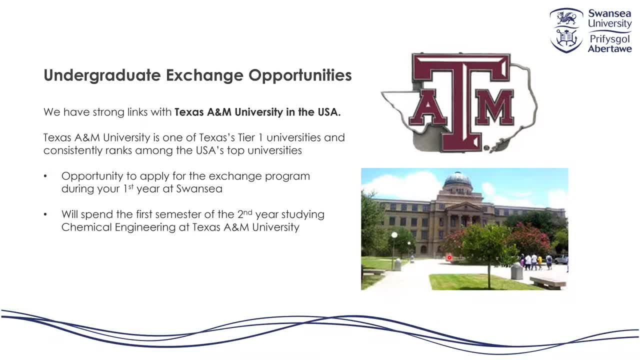 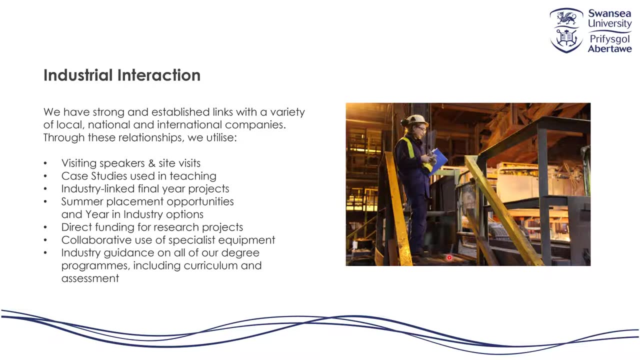 studying there and then you'd fly back in January ready to start your studies in the second semester of the second year, starting in February. One of the other things I'd like to highlight about the degrees course at Swansea University is we have a lot of industrial interaction and links. Our industrial collaborators. 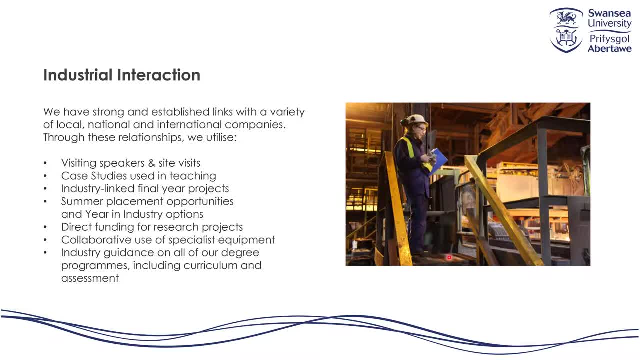 take part in the industrial advisory board, continually feeding back in to us what is expected from industry- Okay, what they all want to see students from Swansea University being able to do when they graduate. So they influence parts of the course. they are involved in setting summer placement opportunities. site visits. 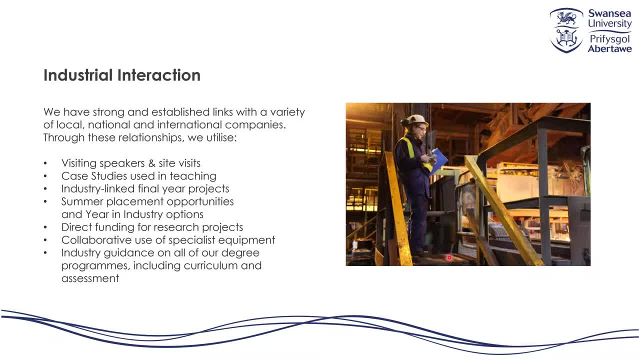 some of them offer offer year in industry options. they even provide case studies for us to use in teaching, and they even come in and do guest lectures for students as well. They also work heavily with our employability team, providing mock assessment centres, e-writing workshops, interview, practice workshops- you name it. Okay, and a lot of this is coordinated. 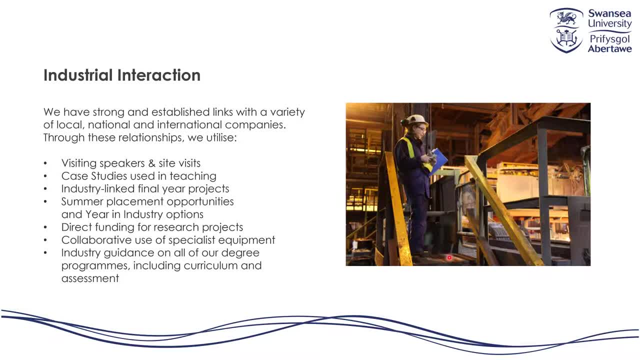 by our employability champion, who actually is an ex-managing director of a company that operates in the South Wales region. He decided to join Swansea University to share his knowledge and experience in chemical engineering, and you'll actually find a link in the description of this video if you'd like to take a look at that as well. 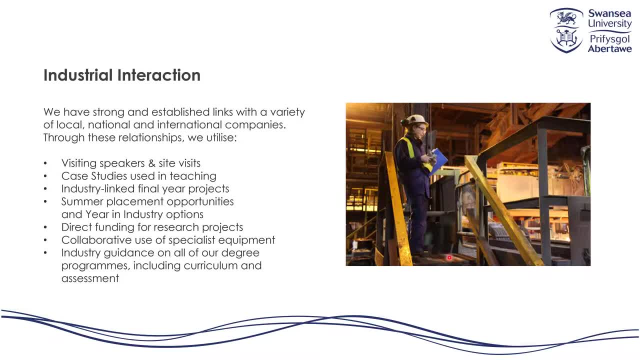 We have a lot of the members of staff who have industrial experience. so we have members of staff who've worked with GlaxoSmithKline. we have a lot who have worked previously in water treatment sectors, membrane separation sectors, things like that. So there's a lot of industrial interaction and involvement in in the degree course. 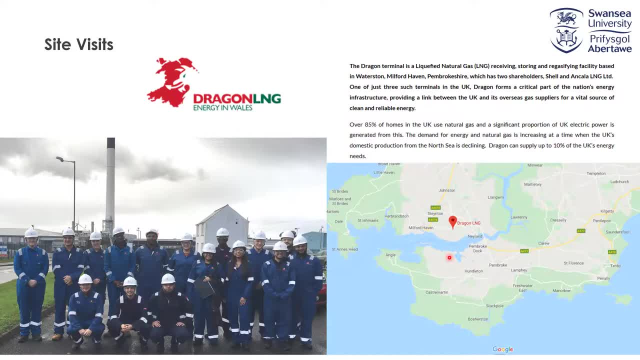 So this is an example of one of the site visits we do. The students were visited Dragon LNG. it's a liquefied natural gas storage facility not far from Milford Haven and South Hook. Our students- you know we like to take our students out and show them the kind of things. 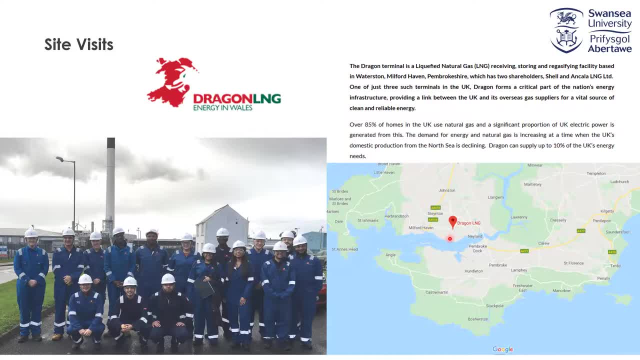 they could be working with and getting involved in. Dragon LNG is one of them. We do take people. we've taken people on visits to places like Gower chemicals across the road. We've taken people to Tata Steel to see where chemical engineers work there. 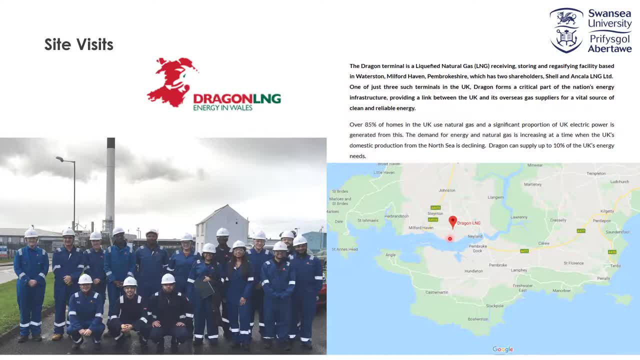 We've taken them to Aberforth power station. We've taken them to places like the paper mill, Cheese factories, You name it. there's a whole wealth of these in the South Wales region. We've even taken them to Dow Chemicals down in Barry. okay, 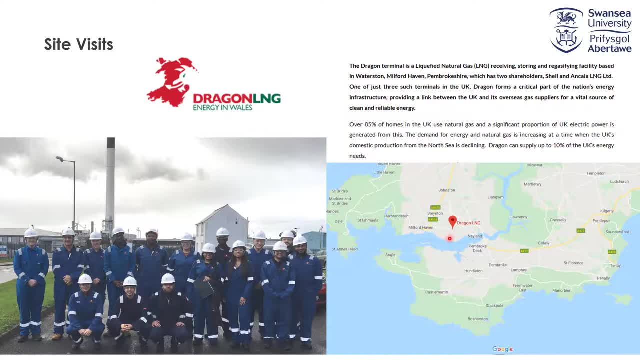 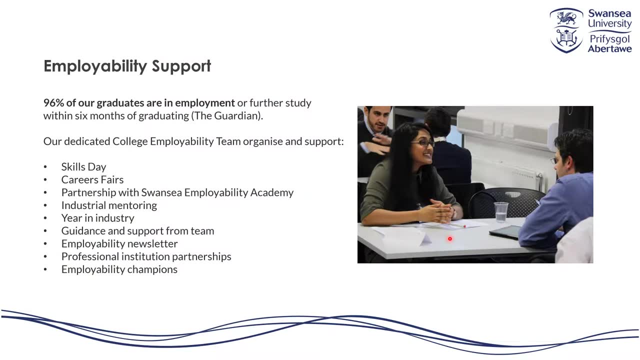 And this is all to give the students experience and an opportunity to see what they could be doing once they graduate. And because of all this industrial interaction, we are really proud of our graduate employment rate. You know, 96% of our graduates for chemical engineering are 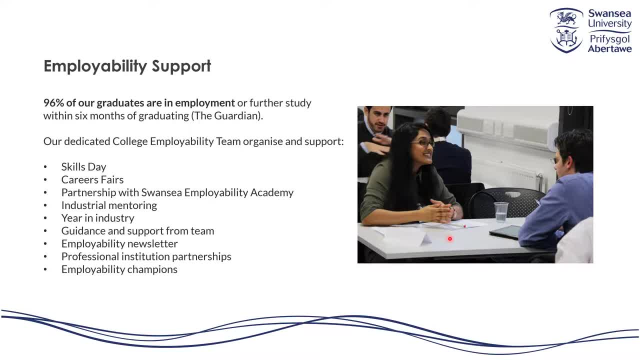 employment or further study within six months of leaving us. okay, And this is because you know Swansea University provides a lot of opportunities to help you improve your employability for companies. okay, Every portfolio. I was included as an employability champion. 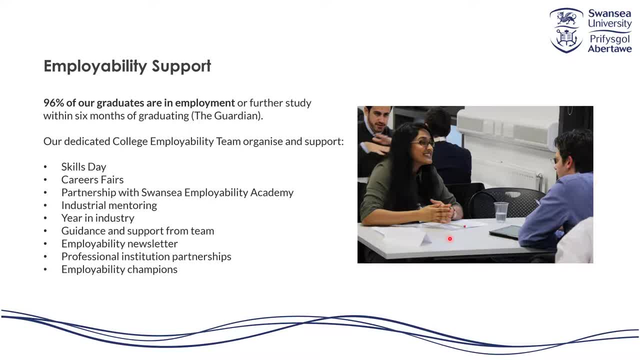 You know regularly running drop-in sessions for CV workshops, we have careers fairs, you name it. Some of the projects that our third-year chemical engineers are involved in have also been set by industrial collaborators and they provide mentoring on those projects as required. okay, 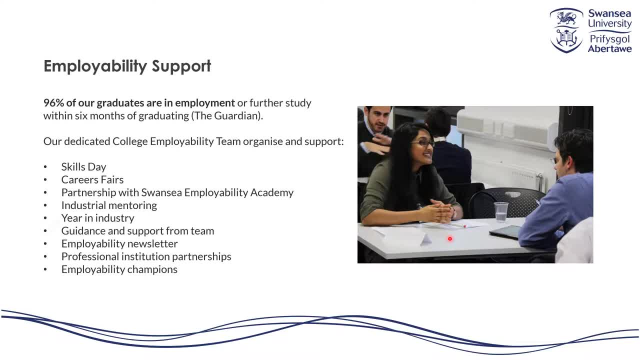 So there is a wealth of opportunities to help you improve your employability. So there is a wealth of opportunities to help you improve your employability. So there is a wealth of opportunities to help you improve your employability. So there is a wealth of opportunities for you to improve your skills.